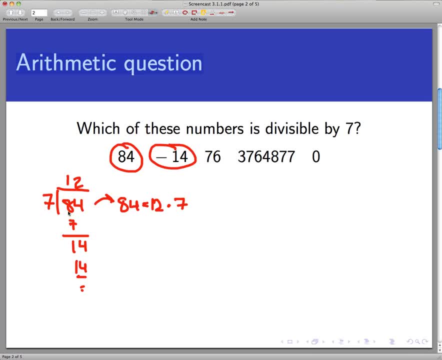 Now, why is that? We don't typically think of having negative numbers in long division And again, naively, we could just pull out a calculator. But can we rewrite it like this: Can we take negative 14 and write it as something times 7? Is negative 14 a multiple, an integer multiple, I should say, of 7? And of course it is because I could fill in that blank with negative 2.. So 84 and negative 14 are both divisible by 7. for the same reason, I can set up this little equation here and write 84 or negative 14.. 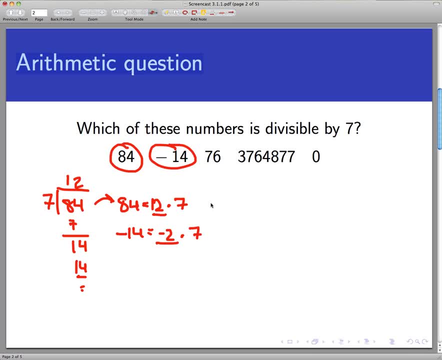 As an integer multiple of 7.. Now what about 76?? Naively again, the calculator way of answering this would tell us no way. that's not going to be divisible by 7.. If I punch in 76 divided by 7, I get a decimal answer. Now what that means in terms of our alternative way of thinking about it is: if I set up, 76 equals blank times 7, could I put an integer into this blank to make the equation true? And the answer is going to be no. There's no integer in this equation that's going to be divisible by 7.. 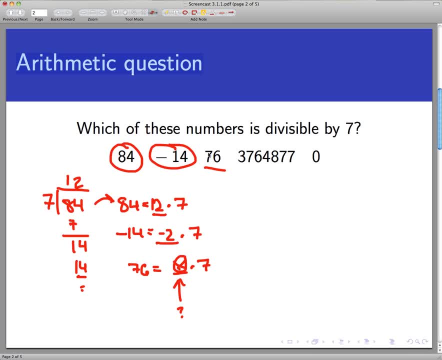 There's no integer that goes here that will make this equation work. So 76 is not divisible by 7.. 3,764,877 is also not divisible by the same reason. If you carry out the long division on this, it's long division. It's quite a struggle, not really a struggle, just a lot of grunge work to get through here. I don't know how many times it goes: blah, blah, blah, blah, blah, And I believe that is the remainder. here you get, You do get a remainder, and it's 4.. So the remainder is not 0.. 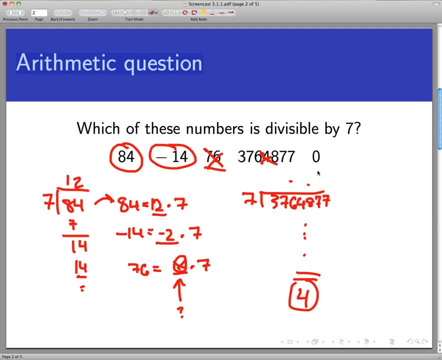 Hence that's not divisible by 7.. What about the number 0?? Is that divisible by 7?? That's a little hard to think about too, with long division somehow, unless we use this alternative way of looking at it. So let's set up the equation: is 0 an integer multiple of 7.. Can I put an integer in this blank that makes the equation true? And of course I certainly can. I can put in the integer 0.. So 0 is actually divisible by 7.. 0 is divisible by 7 as well, because it's a multiple of 7.. 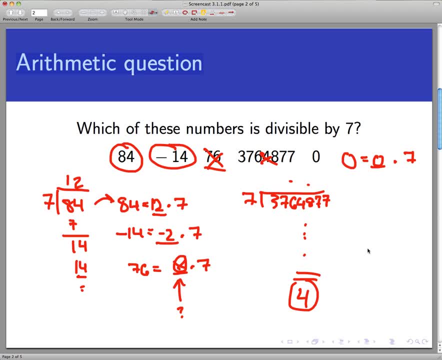 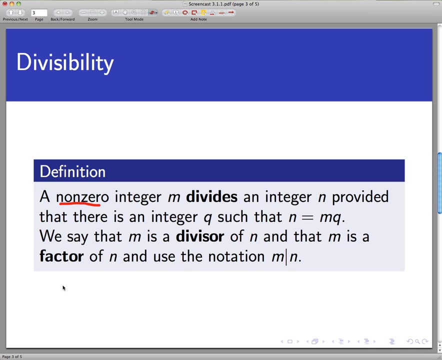 So we're thinking about divisible by 7.. So we're thinking about divisibility in terms of multiplication, which is kind of a nice way to think about divisibility, because division is actually quite a difficult operation to understand. So we can understand whether an integer is divisible by another integer by seeing if it's a multiple of that integer. And that is what leads us to our big definition in this section. We're going to say that a non-zero check that non-zero we never divide by 0 here. a non-zero integer m divides an integer n, provided that there is a multiple of that integer. 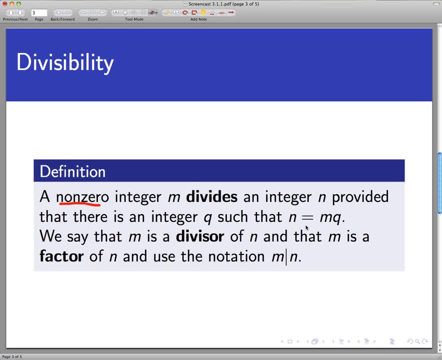 We're going to say that a non-zero check that non-zero. we never divide by 0. here- a non-zero integer m divides an integer q, such that n equals m times q. What this is really saying is that m divides n if n is a multiple of m. Get your n's and m's straight. 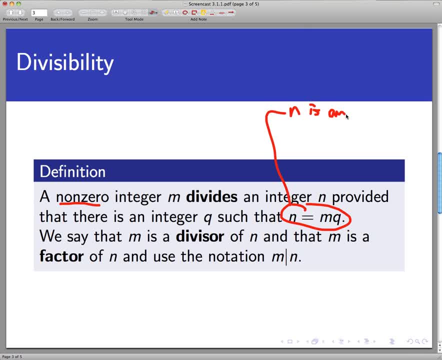 What this is really saying here is that n is an integer multiple of m, Integer multiple of m, Just like 84 was an integer multiple of 7, therefore 7 divides 84.. We also say in some different ways that m is a divisor of n and that m is a factor of n, And then we use this notation: m divides n. This is not a fraction here. This is not the fraction m over n. 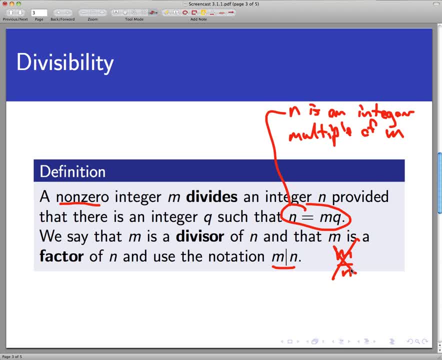 We're actually staying really, really clear of fractions here. We don't do fractions at this point in the course, So this is just a sentence. This says m divides n. Let's look at some examples here of how we instantiate this definition. 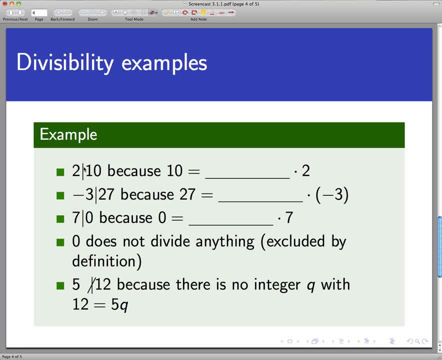 So 2 divides 10, and that's how you would read this: 2 divides 10, because 10 is an integer multiple of 2.. Namely, there is an integer, namely 5, that I can put here. That's the q in the definition. 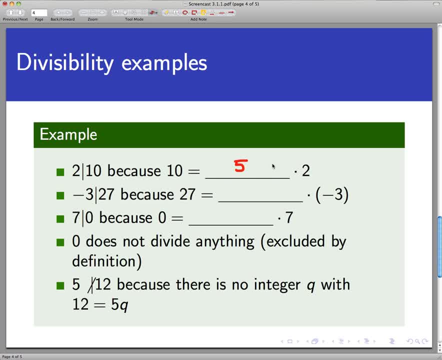 10 is equal to 5 times 2.. There is an integer that I can multiply 2 by to get 10.. Similarly, negative 3 divides 27, because 27 is an integer multiple of negative 3.. I'm sorry, negative 9 times negative 3.. 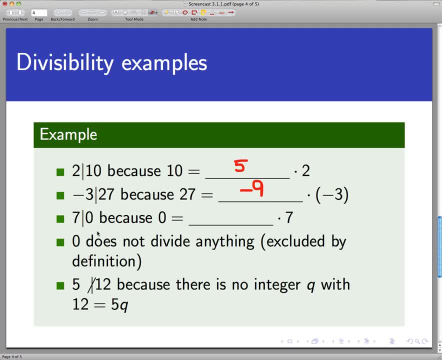 I can write an integer in this blank that makes this equation true: 7 divides 0, because 0 is equal to 0 times 7.. All three of these examples I'm putting in an integer into that blank to make the equation true. 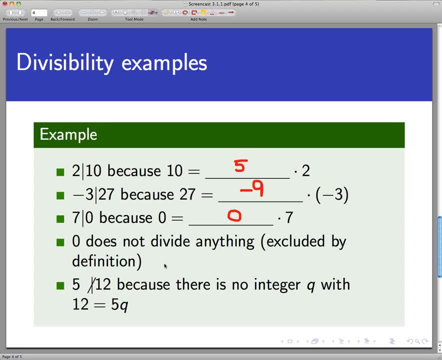 0 does not divide anything. That's excluded explicitly in the definition. Division by 0 is undefined. It doesn't equal anything, not infinity or something crazy like that. Finally, 5 does not divide 12.. That's how you would read that symbol, because there's no integer q, such that 12 is equal to 5 cubed. 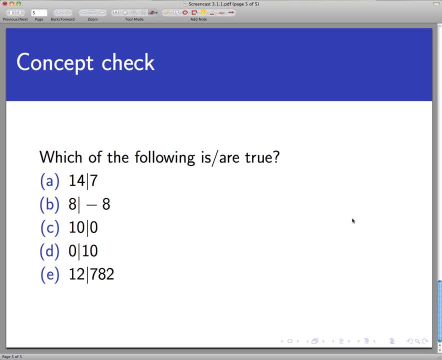 So now it's time for a concept check. Which of the following five statements is, or are, true? You can just pause the video and select all that apply. Okay, now that we're back, let's just tick down the list here. This is not true. This says 14 divides 7.. 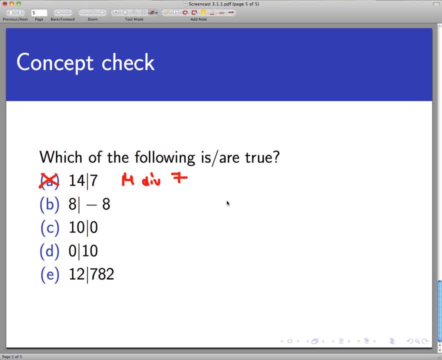 14 divides 7, and that's not true. The other way around would be true: 7 divides 14.. If 14 divided 7,, then I would have to be able to fill in the following blank with an integer. Now I could put a fraction in this blank, namely the fraction 1 half, and make this true. 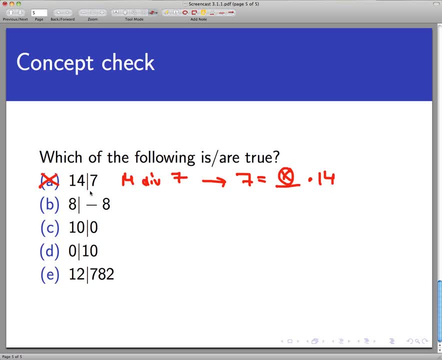 But there's no integer. There's no integer that goes here. that makes that true. So 14 does not divide 7.. However, 7 does divide 14.. So this is a one-way kind of operation. 8 does divide negative 8.. Why? 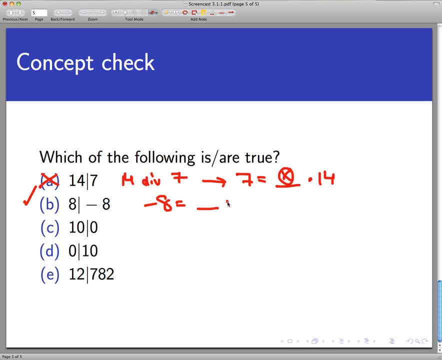 Because I can take negative 8 and write it as some integer times 8.. Namely, I can put in the integer negative 1 into that blank. So this is good: 10 does divide 0. We've seen a couple of examples of that already. because I could take this equation, set it up and put an integer in this blank, namely 0. 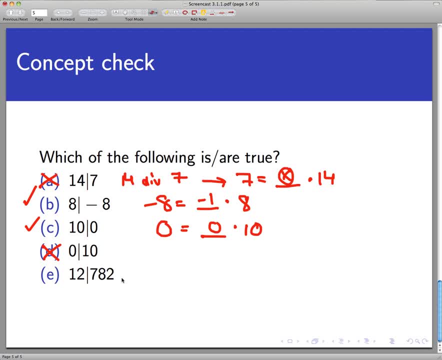 This is not correct, because 0 does not divide anything. Does 12 divide 782?? Well, so we can determine whether 12 divides 782.. One way to do this is by writing out multiples of 12.. What are those multiples of 12?? 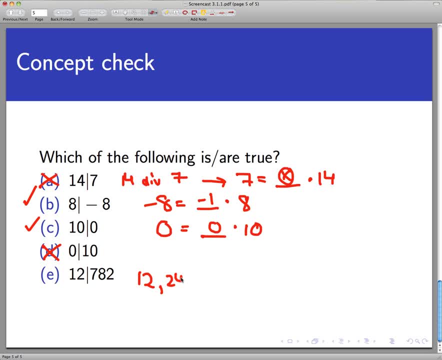 If I start with the positive multiples of 12,, I'd have 12,, 24,, 36.. Let's make a list of these guys here: 48.. Let's skip a bit and we will eventually, after a long time, after 60 of these, end up at 720.. 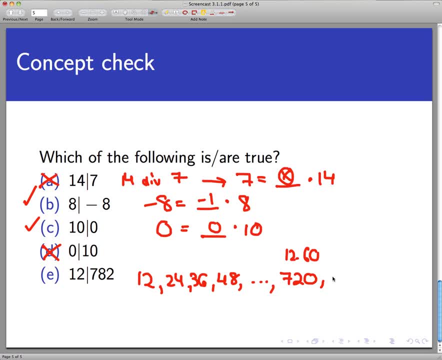 That's 12 times 60.. Let's keep going from there: 732, 744.. And what I want to do is see if 782 shows up in the list of multiples of 12.. This is slightly an inefficient way to do this, but it will become helpful for us in another section where we talk about integer congruence coming up.